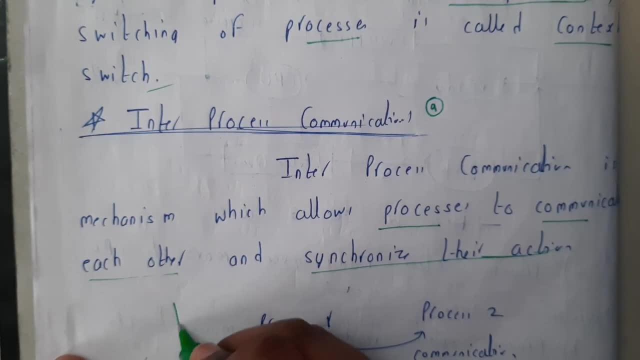 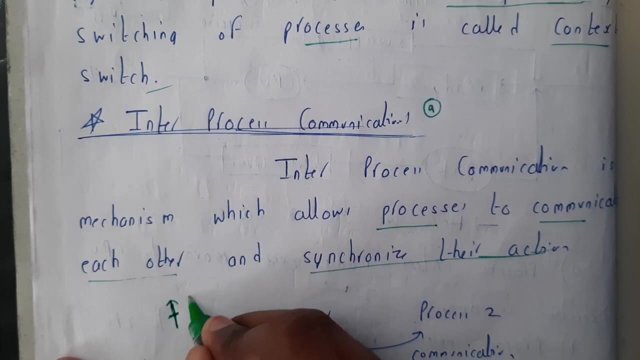 first, or okay, let us assume that there are two processes, They need to execute 100%. So initially the first one did for 50%. So it is giving the chance for second process to do 50. Then this will be done. this will be done. So this is nothing but with inter-process. 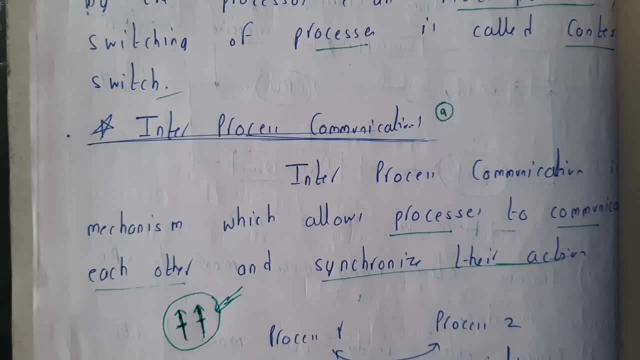 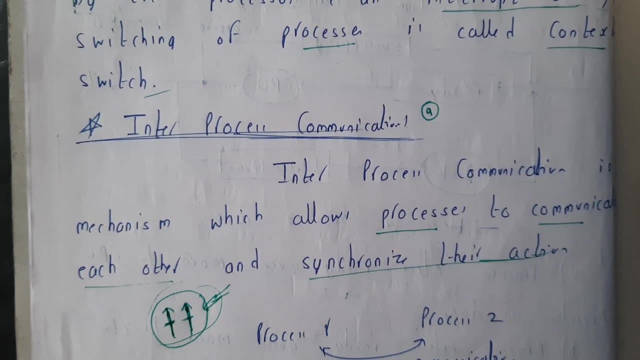 communication. they are understanding themselves And they are doing the works Right. So inter-process communication is a communication which they can communicate each other, synchronize their actions. So in this way they can synchronize their actions. So process one, process, two Communication, This is nothing but inter-process. 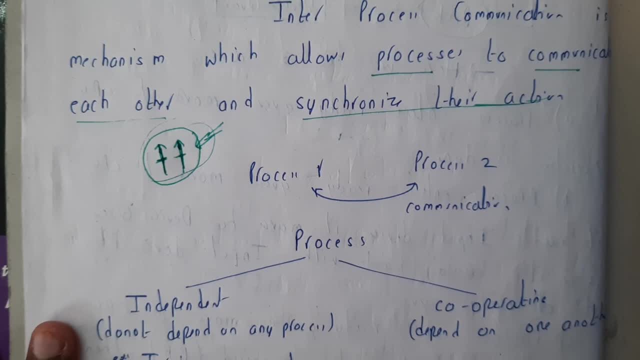 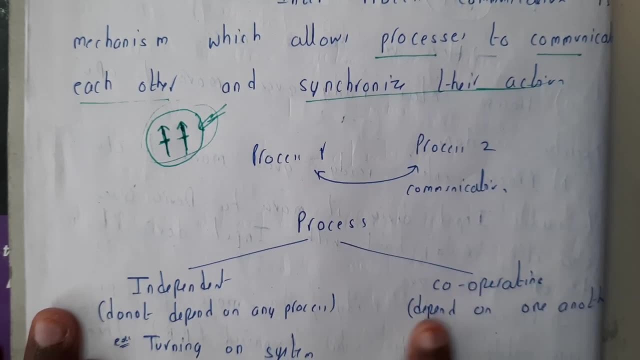 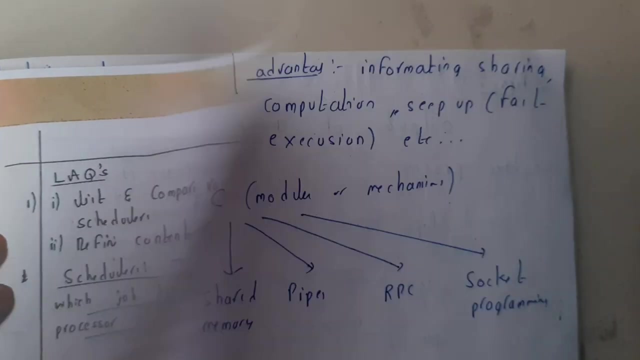 communication. So basically, processes can be divided into two types. One is independent process. Basically this do not depend on anything, Whereas cooperative processes, these depend on others. So here we can do this inter-process communication perfectly. So basically, you may ask me that what will be the advantage? 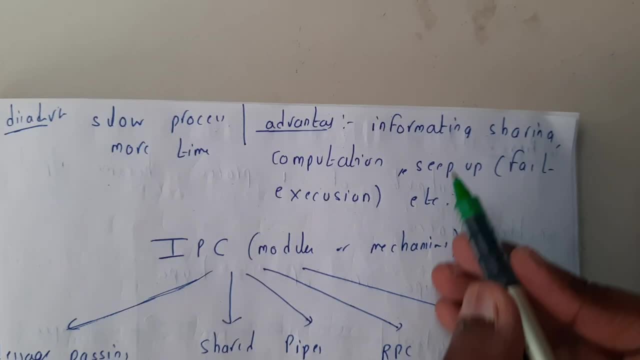 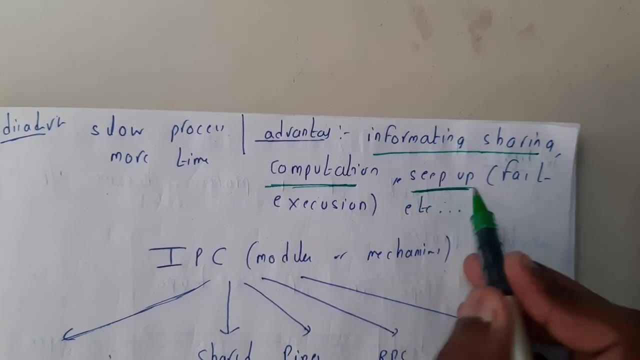 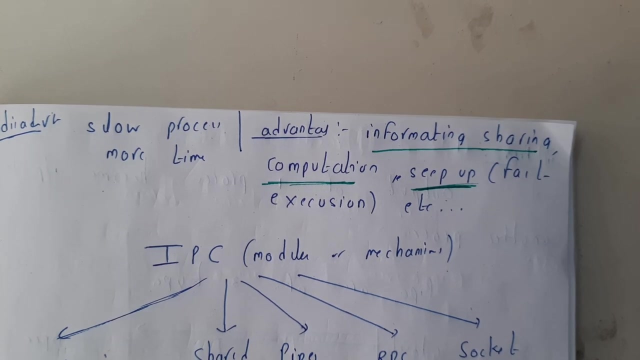 if we do this inter-process communication. so basically the advantages will be: we can share the information between the processes. we, the processes, can communicate with each other and speed up. that is nothing, but there can be a fast chances of executions and many other things. so what will be the disadvantages? so the disadvantage will be if there are n number. 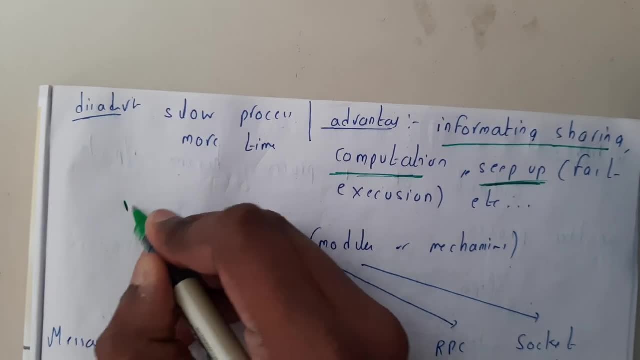 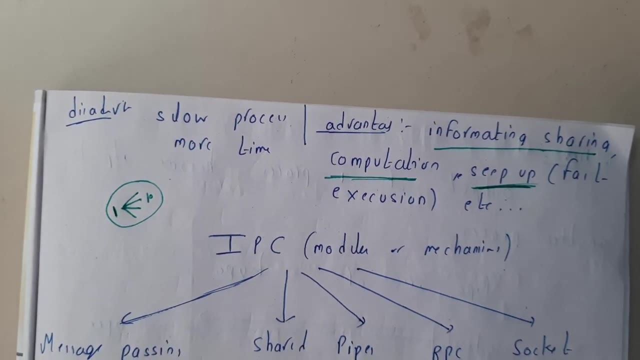 of processes depending on n number of processes. there are five. there is a single process which is depending on 10 processes, so this could be a issue, right? so like this, it's going to make the processing really slow. like that, it takes more time. okay, guys. so now i hope everyone got. 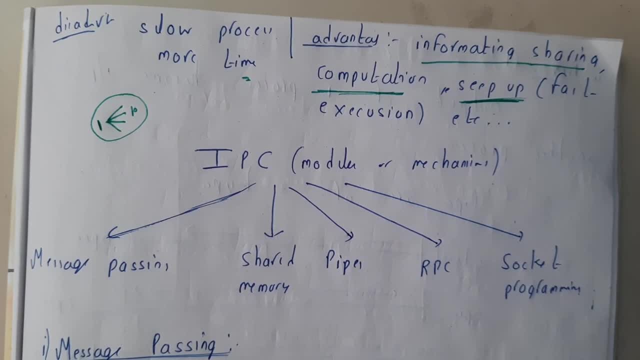 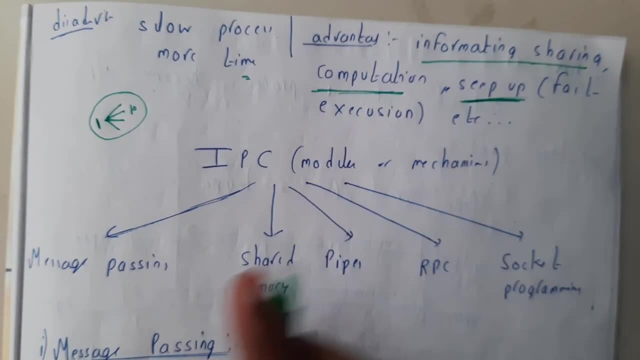 a small idea on this. so now let us continue with. what are the ipc mechanisms, inter-process communication, in how many ways we can do so? there are mainly five types, guys, in this. the first three types are really easy and important. the rest two, which you will be just going through it, don't worry. 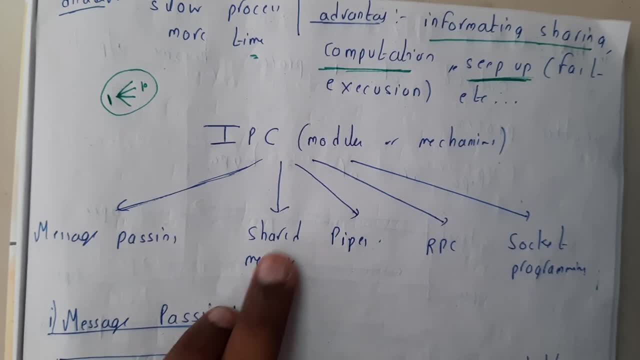 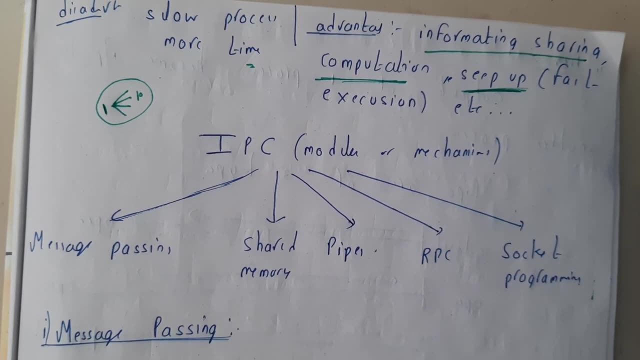 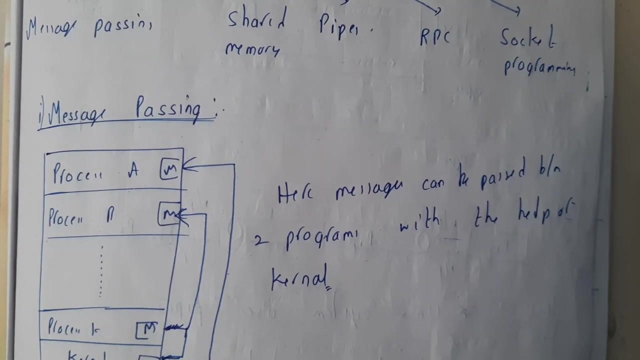 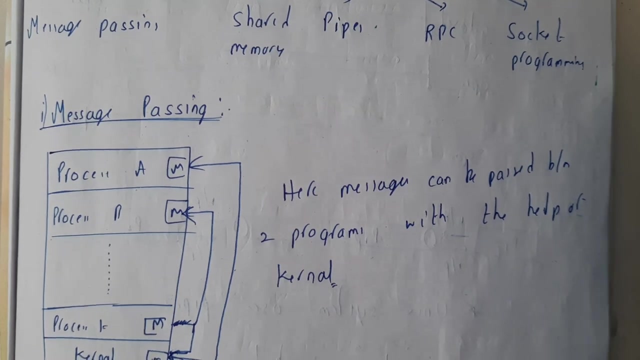 okay, so basically message passing, shared memory pipeline, rpc, remote procedure, communication, call, socket programming- okay so, message passing. so, like our whatsapp or any kind of application, what is message passing? guys, we'll be passing the message to us from our side to the friend side. fine, okay, so basically here we'll be thinking that the message is directly going, so it may or may not. 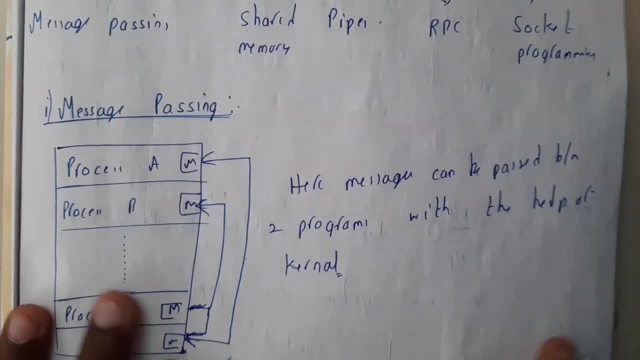 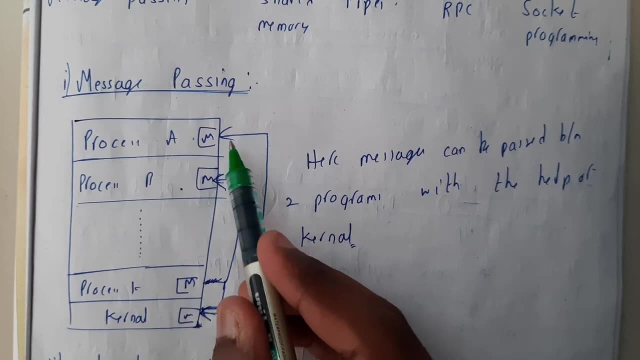 be go may not go in that way. i have no, i have no clear idea about that. but basically in terms of processes, basically if process a want to send a message to process b, so the message from here it will travel, okay. so the message will be sent to the process b and the message will be sent to the 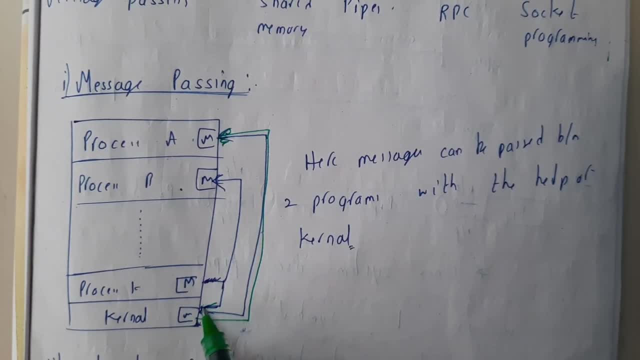 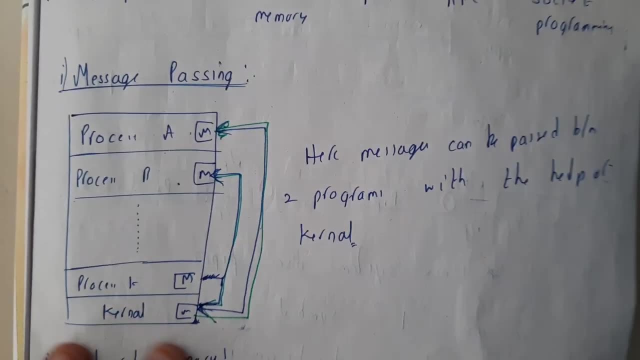 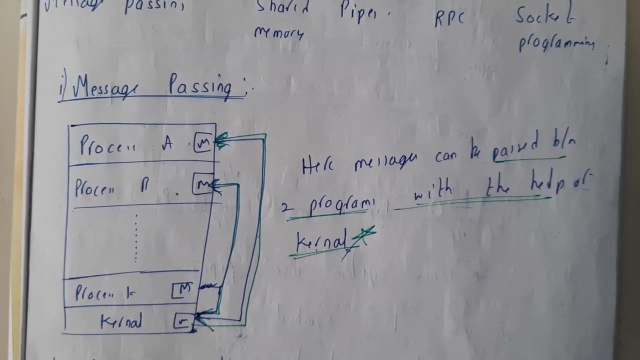 approval. okay, let me correct the arrow. so it will be going in this way, and from the kernel it will be sent to process b. so here the pro. the message passing mechanism will work in this way. so here messages can be passed between two programs with the help of kernel. fine, so only with the help of. 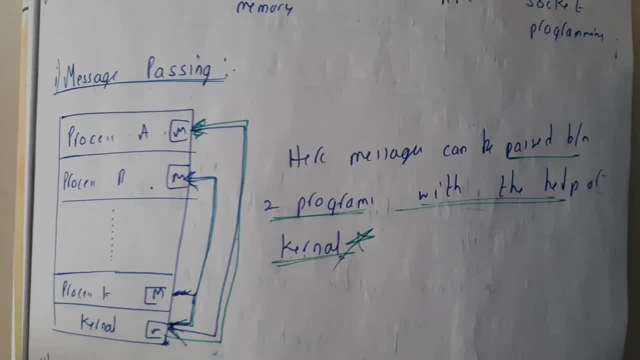 kernel you can do this message passing okay, so message passing in our record. we did a program. so basically in the first program we wrote we it will be taking an interface to our program and finally it will receive an input from our container. so this is what it will do. let's go to our rtmcom. then if you want to struggle with rtm is just you need to manage your rtm table. so basically, 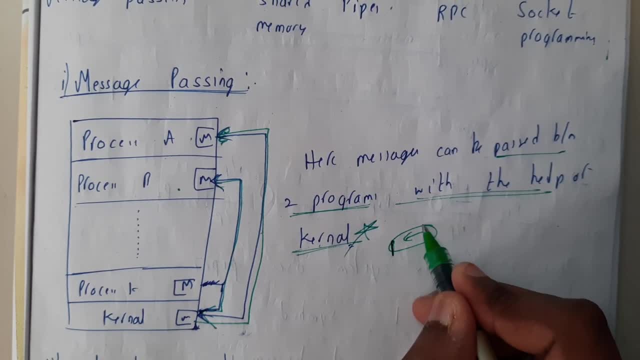 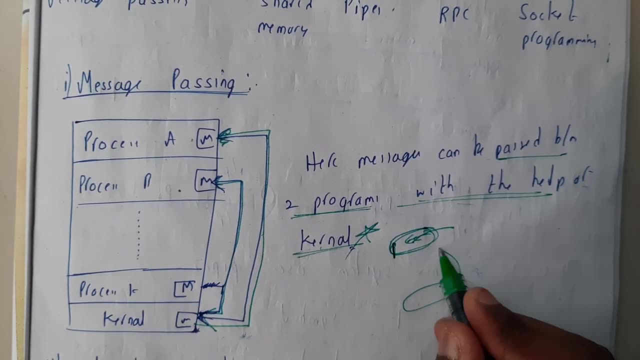 first program we wrote we it will be taking an input of a string. basically we used a shared memory also in it, so it will be taking an input of a string. and the second program will be trying to read this message. so this is nothing but message, message passing. so basically, where these programs are stored in the 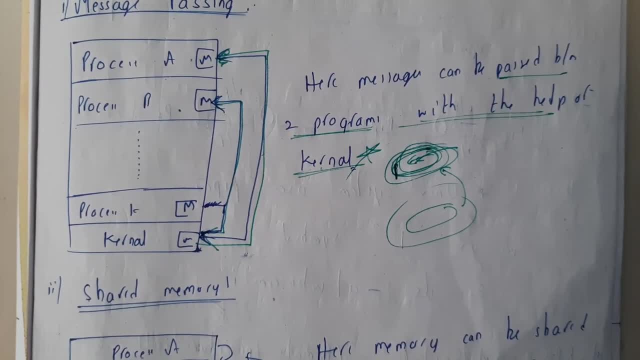 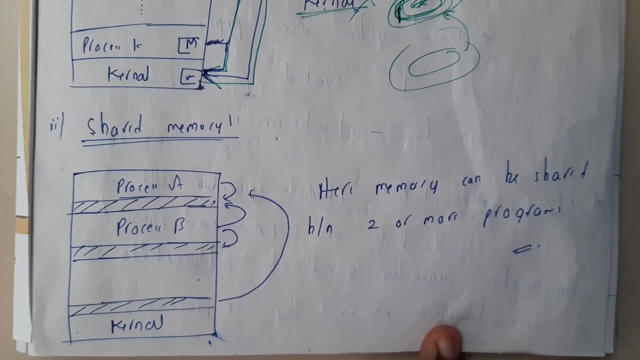 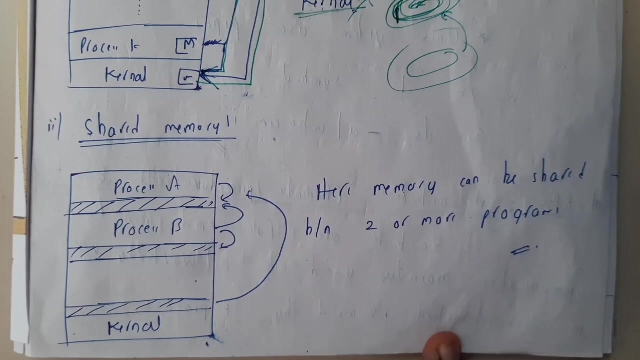 kernel, so that's it. so that's the reason why we will be saying: with the help of kernel, okay. so now let us go through shared memory. so shared memory is nothing but a block of memory space of one process is a shared with another process so that they can use the common variable. so let us assume there are. 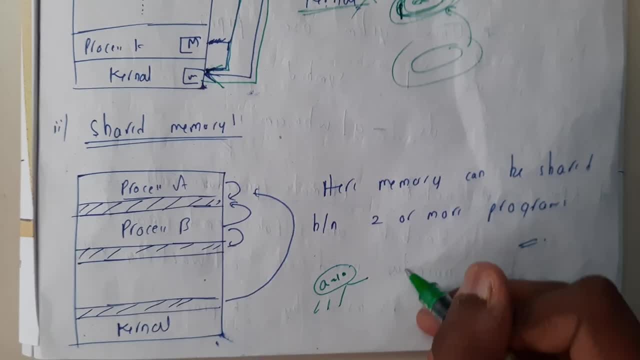 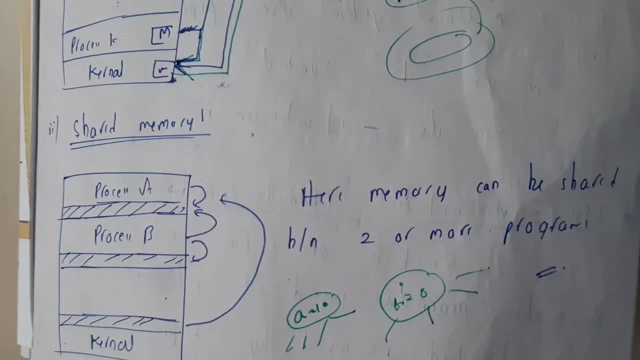 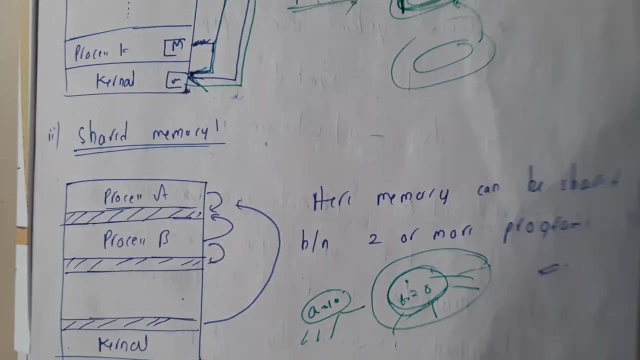 variables: a equal to 10, which will, which we can use in multiple programs, or I equal to 0, which is a common iterative, iterative character which we use for loops. I will do while for that all things will be using right, so we can define it and we can share this to all the processes. so in this way we can use. 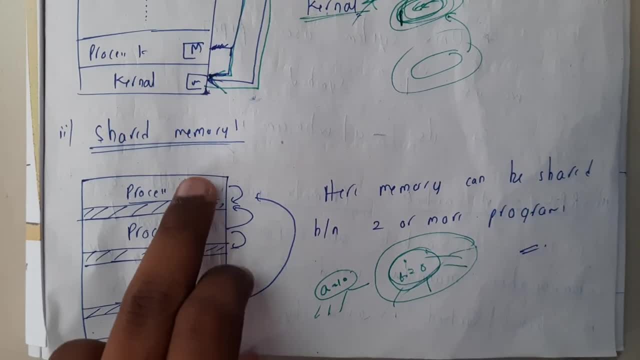 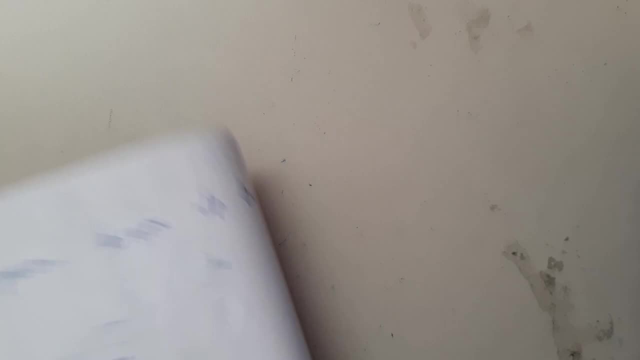 the shared memory. so this is a block of memory space of one process is a shared memory concept. so here the shared memory can be between two process, or kernel and process. in both ways it is possible. fine, so now let us continue with the third topic, that is pipeline. so basically, what is pipeline? so pipeline? 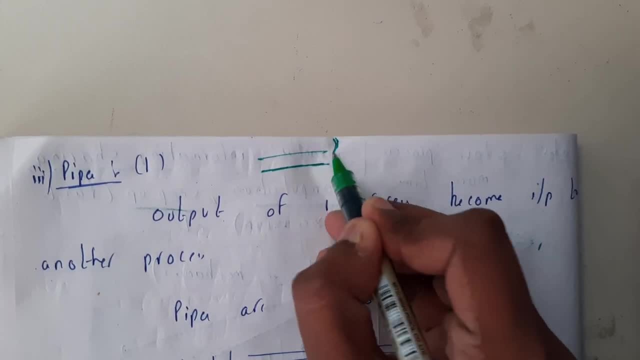 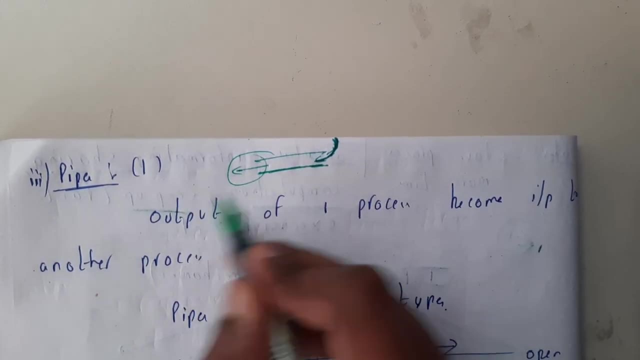 will be something like this. so in in terms of our household, pipelines will be calling water pipelines. so if we connect it one side, it will give the output from the other side. so this is water. this is water. it is traveling, for traveling from one place to another place. 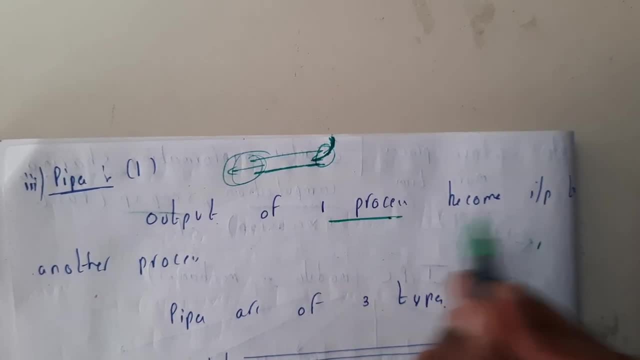 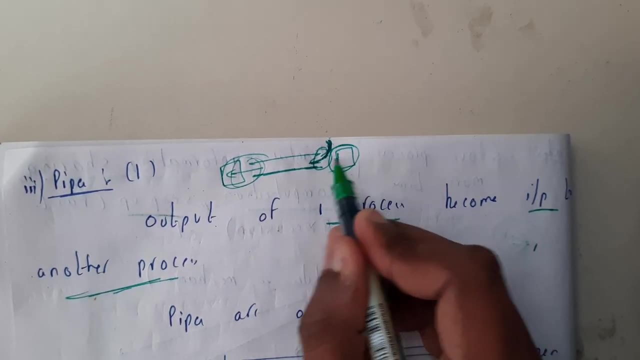 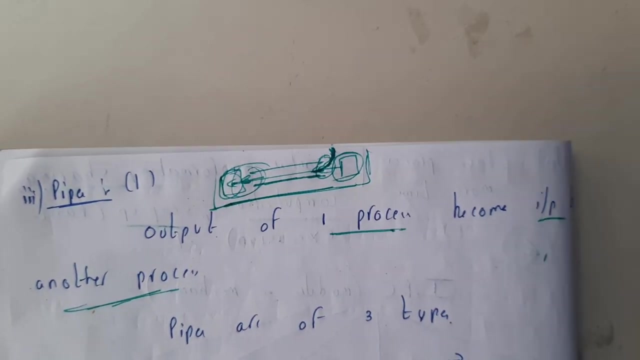 will be using this pipelines. so output of one process becomes the input of another process with the help of this pipeline. so if there is a process here, let us assume, if there is a process here, so this process, output is given as input, right input to this process. so this is the concept of this pipes. in say in: 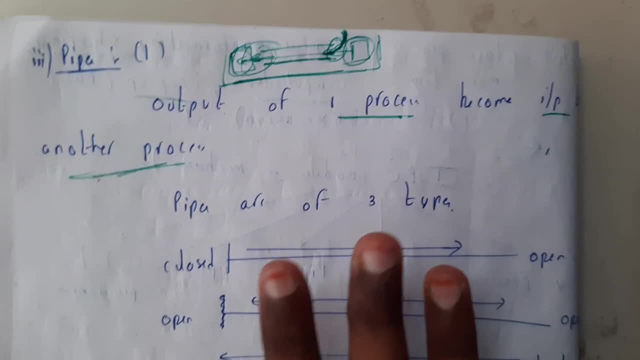 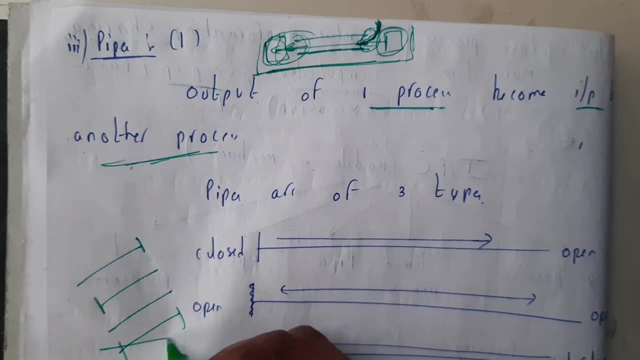 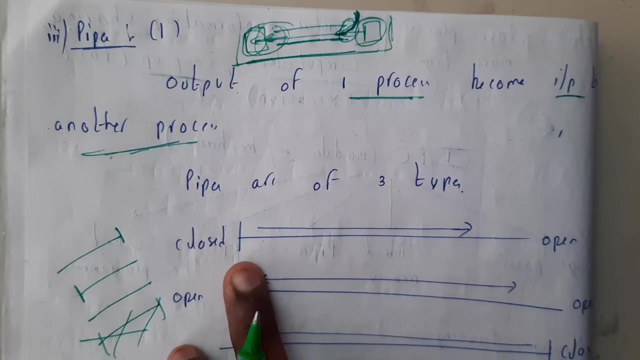 inter process communication. so basically there could be three types of pipes, guys. so basically you can say it blindly: so one side closed, this opposite side closed, two sides open. you cannot say two sides closed. so if two sides closed, what is the use of that pipe? will there be any use? no, so that's the reason why we'll be having a closed, so this: 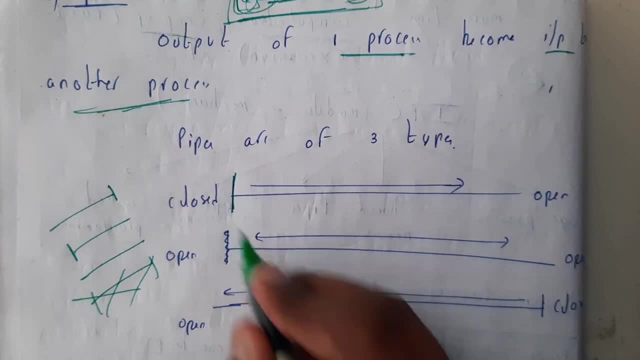 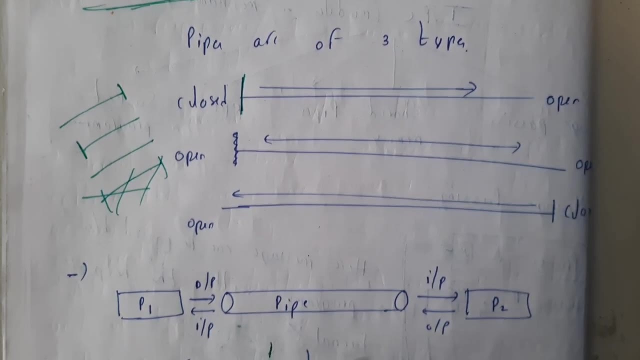 side it is closed and this side is open. so wherever it is closed, you will be just drawing a straight line. wherever it is open, you will be placing an arrow or open end, fine. so this is open, open, this is open, close. so in this way, so how you may, you may ask me that, how we can draw, 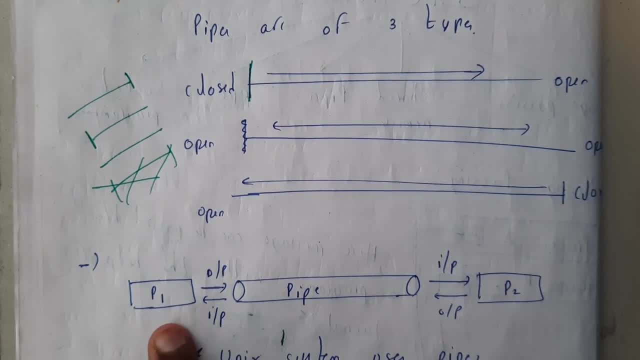 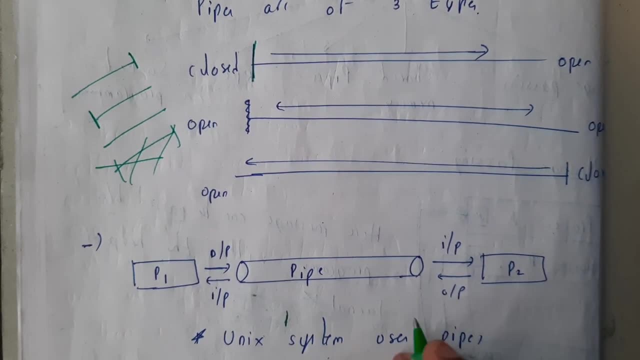 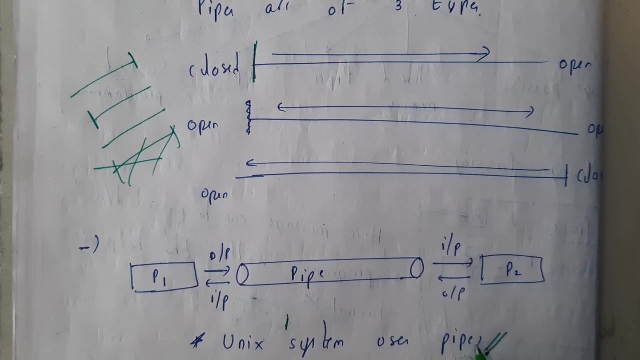 this diagram really clearly. so you draw a pipe and place process p1, that output is depending on this and this output is depending on this. so this is a cyclic process, something like that. okay, so basically, this pipelines are mainly used in Unix operating system, Unix or even Linux also. it is. 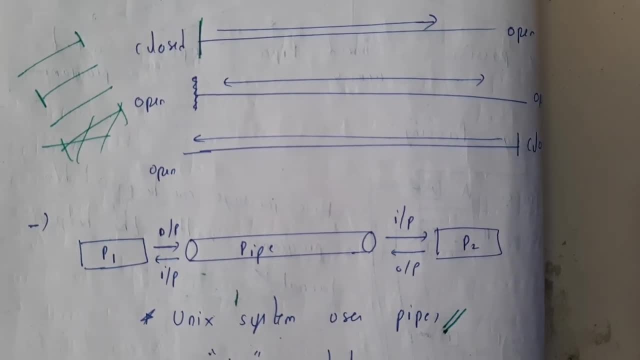 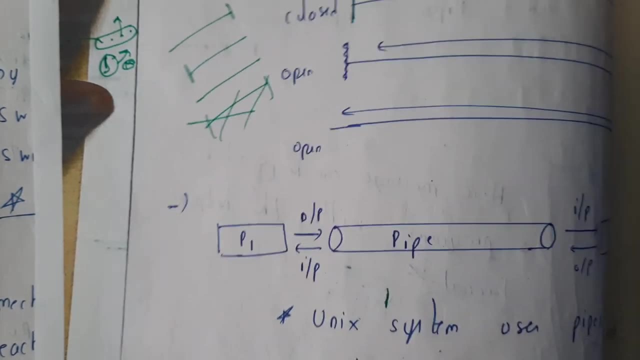 brought to Linux also. so basically, you may ask me that what will be the use of this pipeline? so pipeline is nothing, but we can do two operations. the first operation, output, is given as the input to the second operation. fine, so we use this symbol. I hope everyone can recognize this, or in some 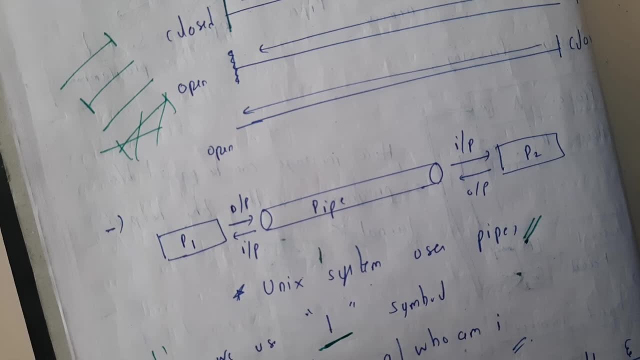 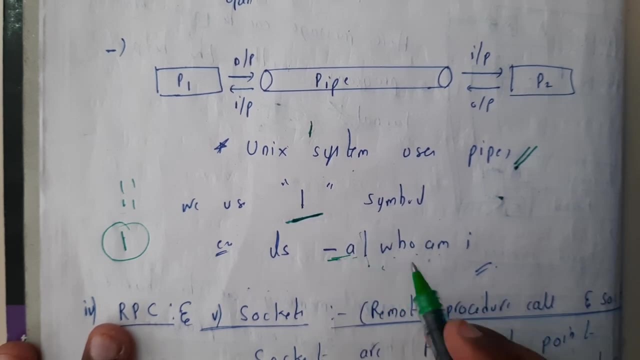 languages. we will be using this, basically. so this in this: we will be using this as an or okay, this is an example for a. we will be using this as an or okay, this is an example for a. so now we will have to do something like this. so let us call. this process will be called remote procedure calls. 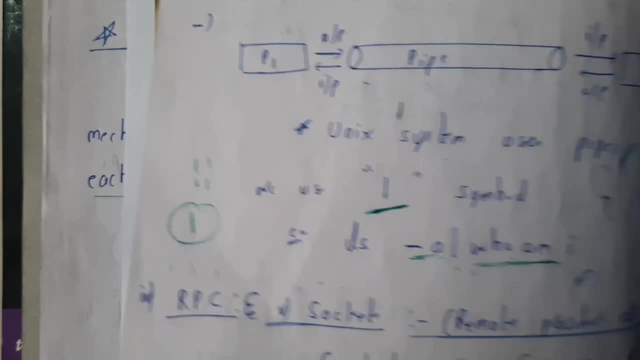 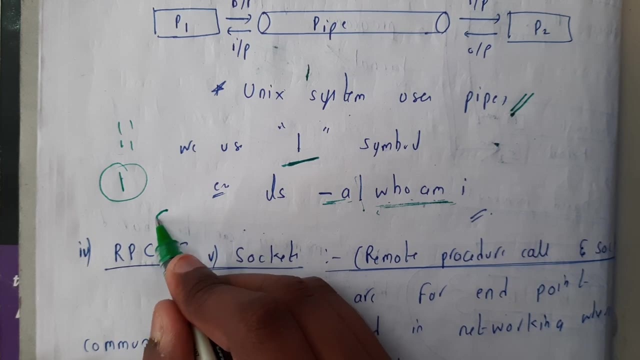 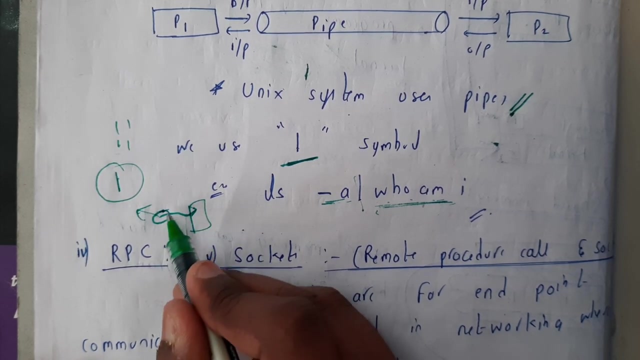 so what is a remote procedure call? the code is written somewhere else and in a program you will be trying to call it. so this is nothing but shared, right? so we are communicating with some other project of another project in some part to the other part. so that is a really nice structure. of the process. so in one of the case this is a simple procedure call. so that is what I am going to do. for once, I say I am going to call, it is to promote the program, so if I want to call it, then I am going to call it.